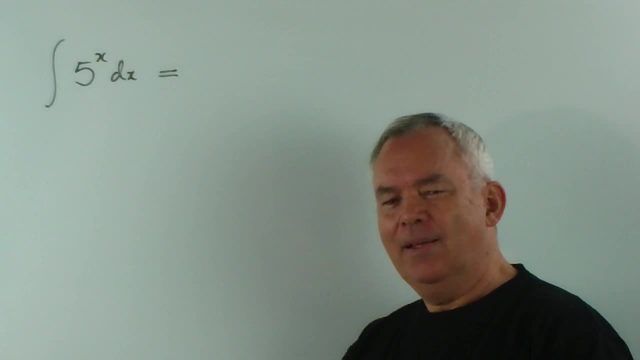 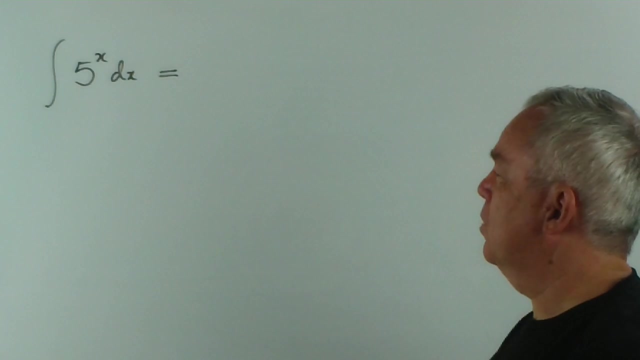 G'day. This particular integral obviously does not involve trig functions and it's not a power of x. It is in fact something to a power of x, which is an exponential form, But sadly it's not either the power x And this particular kind of integral disturbs. 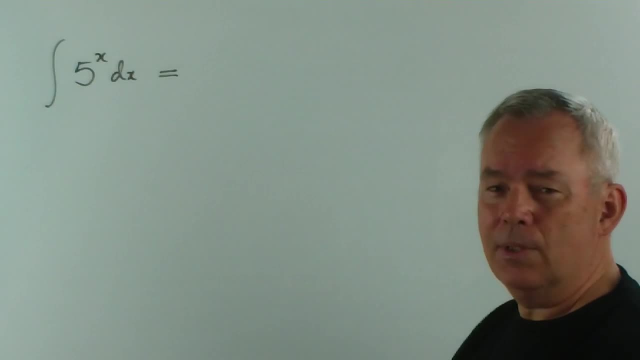 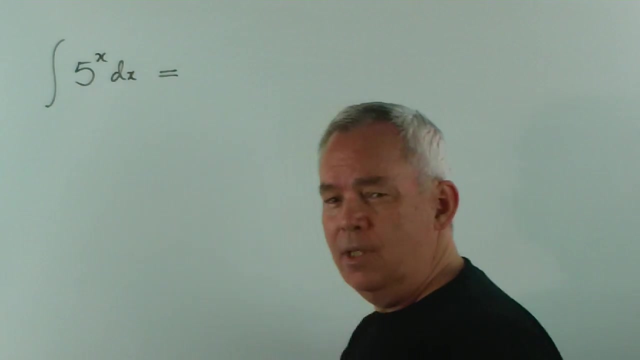 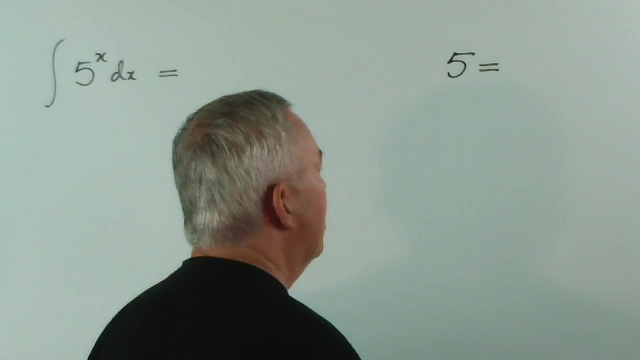 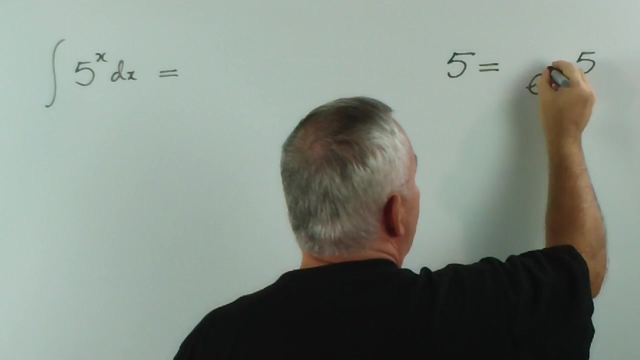 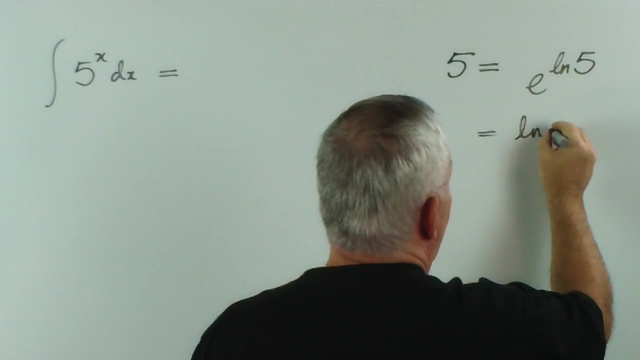 lots of students. I want to show you what to do with it, to solve it fairly quickly. To solve it, we need to replace this 5 with an e, And we need to do that. we need to understand something. 5 is the same as e to the log 5.. For that matter, it's the same as log of e to the 5,. 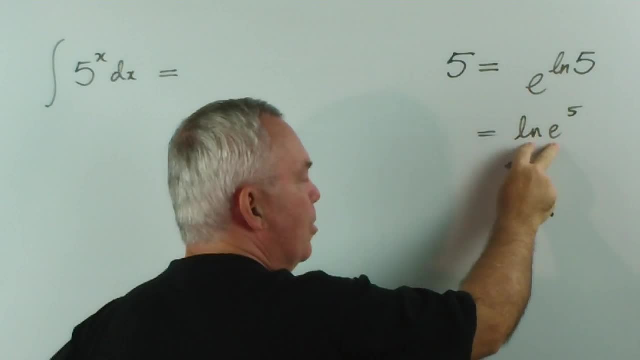 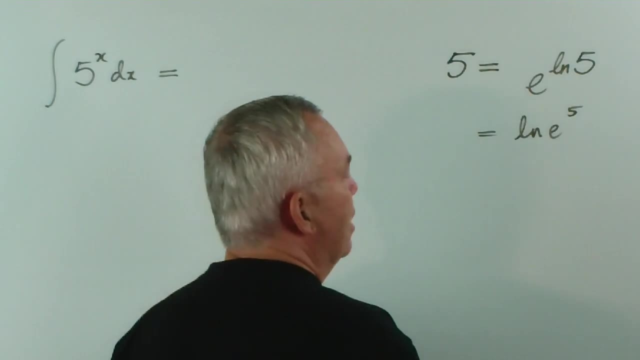 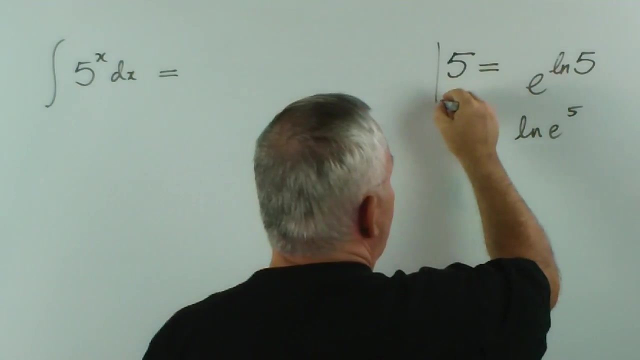 for the simple reason that exponential functions and logarithmic functions are inverse functions, And this undoes that, Or this undoes that. So 5 equals 5, 5 equals 5.. Which substitution will be useful for us? It'll be this one. You just need to know this trick. 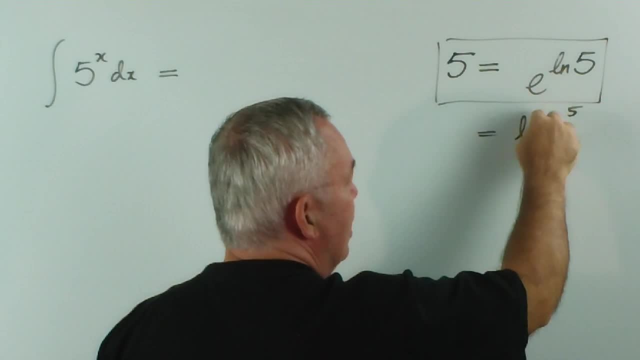 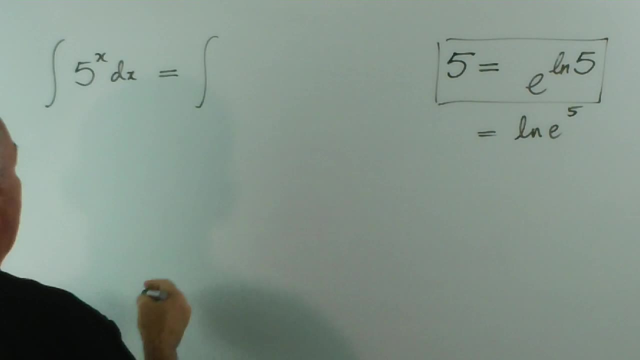 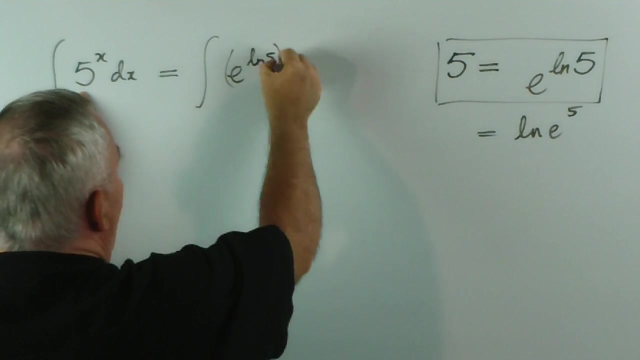 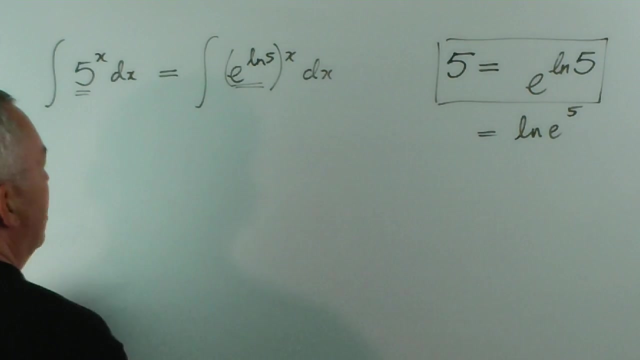 that any number, if you want to convert it into an exponential, is the exponential of the logarithm of that number. We've become replacing the 5 with e to the log 5, all to the power, x, dx. So all we've done now is replace that 5, using our knowledge of inverse functions. 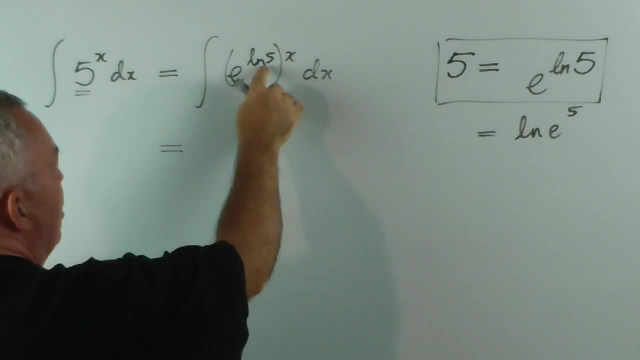 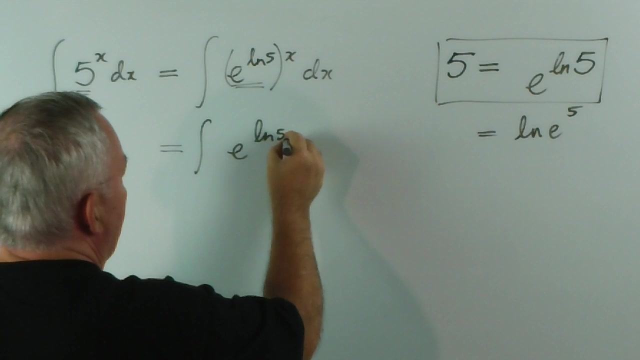 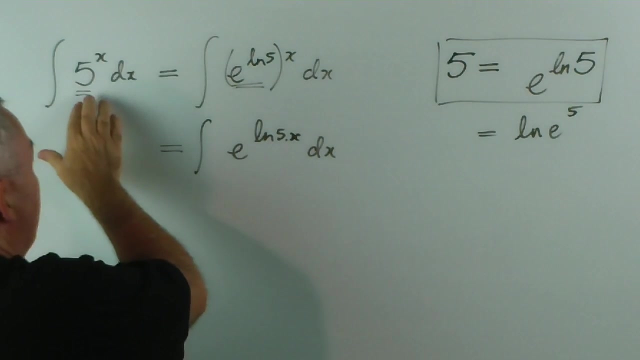 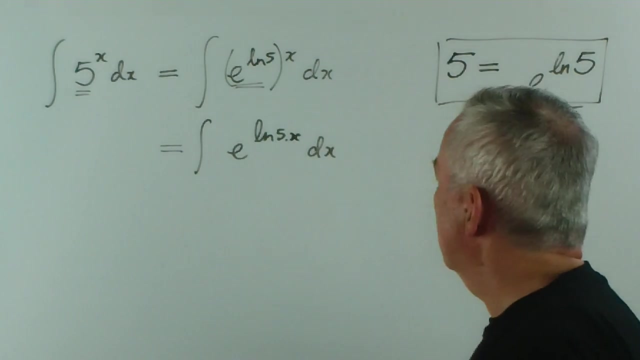 When you have a power of a power of e, you multiply the powers, So this is the same as the integral of e to the log, 5 times x, dx. Now we've succeeded in converting this exponential into an exponential involving e, which is our preferred form. 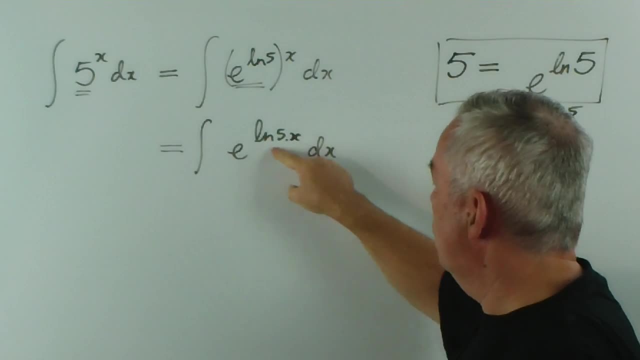 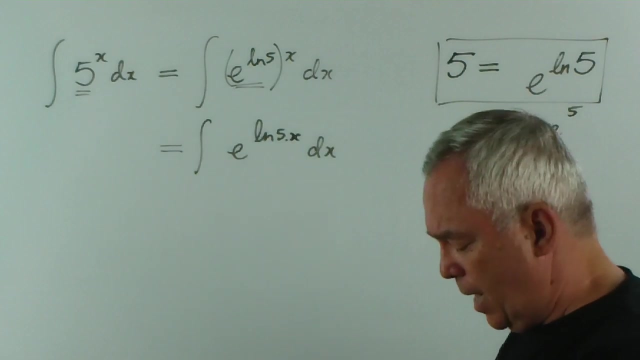 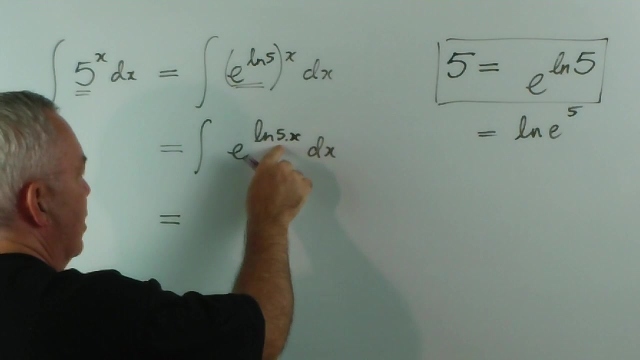 Now, how do we perform it? We could substitute u for that, but I think you've seen by now that for a lot of these simple ones, I'm trying to follow a pattern, And the pattern is this: That if you add e to a function of x, then 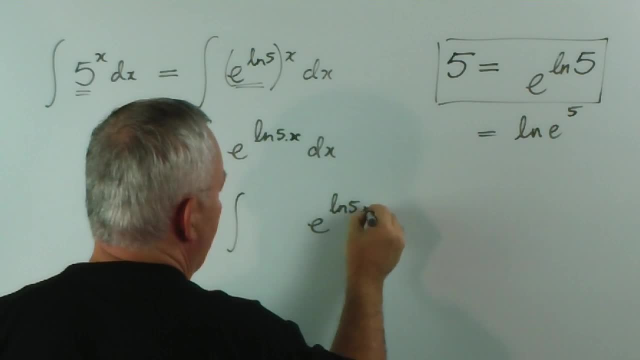 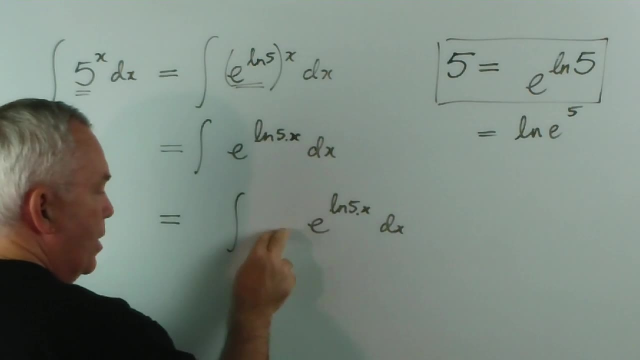 well, let's write this out. we want, in our pattern, to have the derivative of this here. Now, the derivative of that. since log 5 is just a constant, it's just like 2x or 3x or 7x- the derivative of this is log 5.. 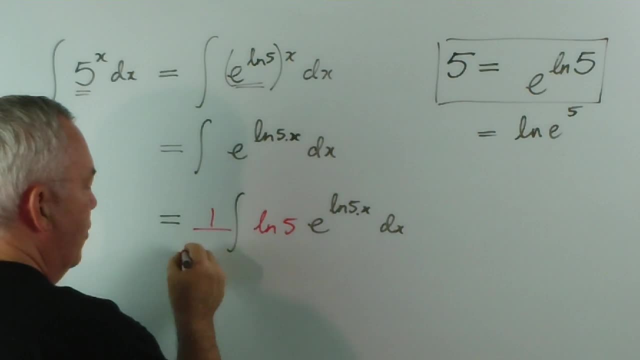 And of course, to compensate for putting that number there, we divide by log 5 out the front or multiply by 1 over log 5.. Of course that times that is 1 and again multiplying by 1. 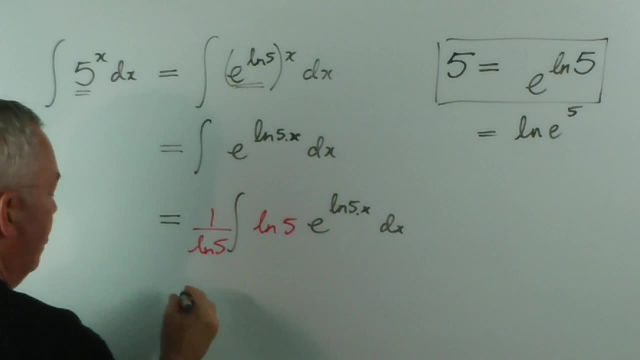 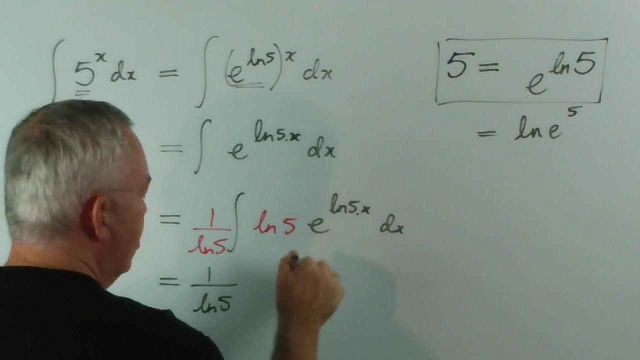 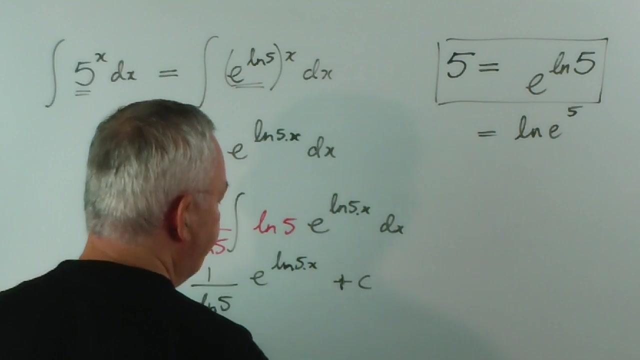 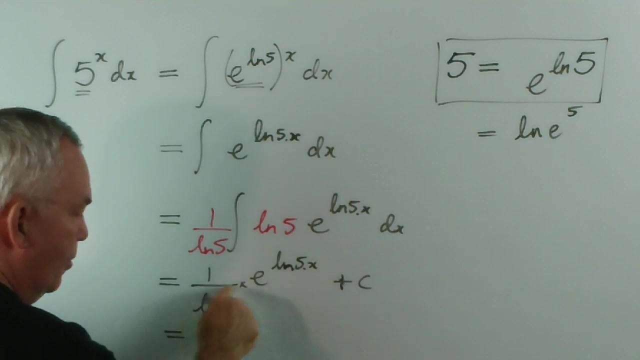 makes no difference to the value of the integral. Therefore, we get 1 over log 5, and the integral of this is just that function plus c. Now, of course, because this is a fraction multiplied by this, I can write 1 times the exponential over the log 5. 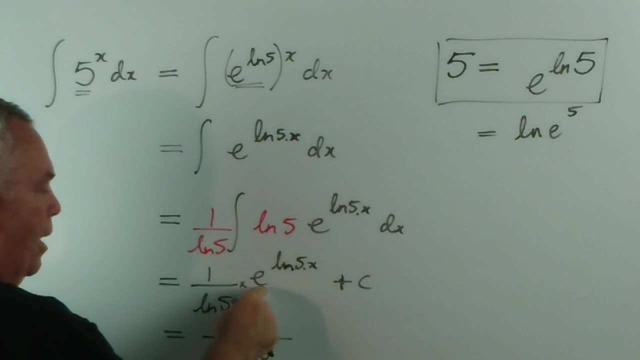 so I put the log 5 on the bottom And remember exponential to the logarithm of 5 is worth 5.. So it's just back to our 5 to the power x, Remember the x remains. We've just changed that back into a 5.. 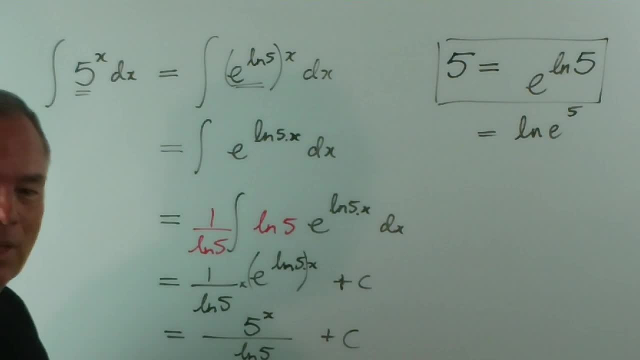 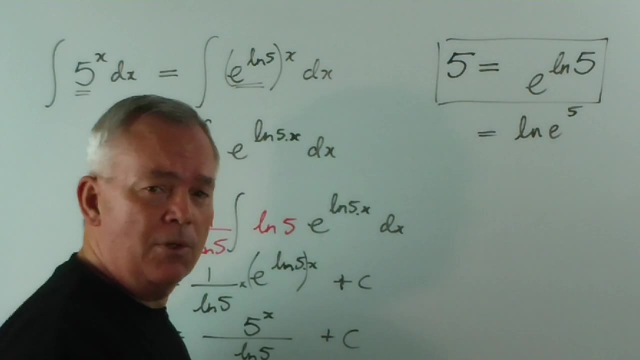 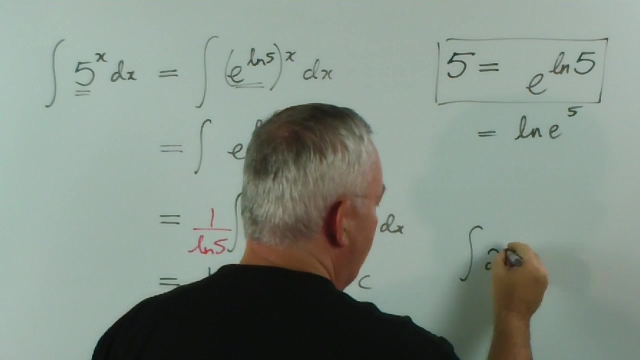 So slightly unusual, a slightly nasty little kind of integral. As long as you understand how to use your inverse functions, you should be right, And if you memorise this pattern you'll realise a useful pattern to work on is that some number like 29 to the x dx. 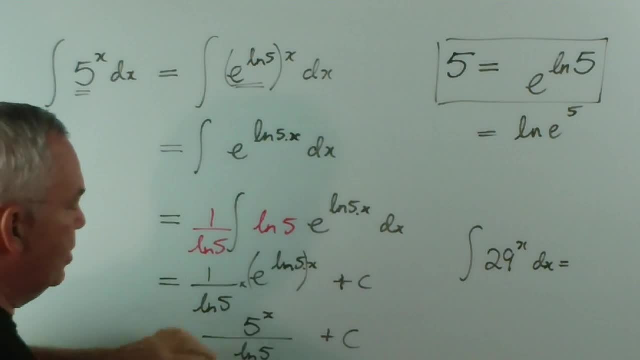 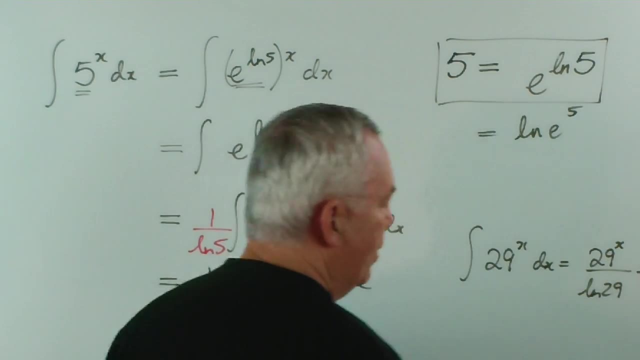 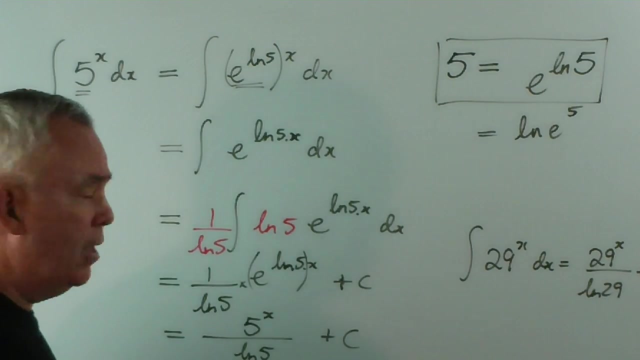 when you integrate it is going to look exactly like this: does 29 to the x on log 29 plus c. Now again you can go through this process. it's very worthwhile doing, by the way, a few times to practise these kinds of conversions and substitutions.